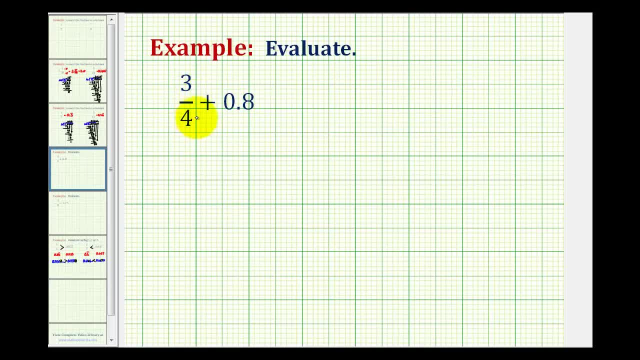 to a decimal. Remember this fraction bar means division, so to convert three-fourths to a decimal, we'll divide three by four. There aren't any fours and threes, so we'll add a decimal point, move it up to the quotient and then add a zero. 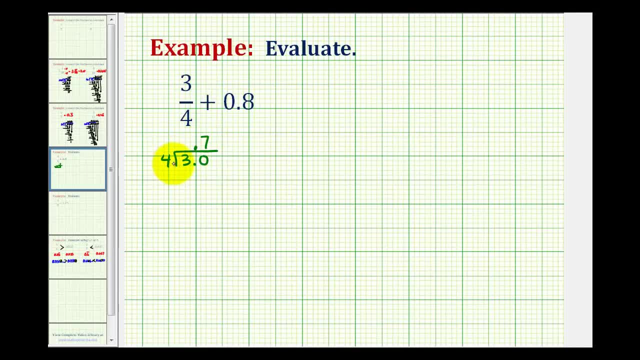 Now we want to know how many fours are on thirty. that would be seven. Seven times four is twenty-eight. This difference is two. Add another zero and bring it down. Now we want to know how many fours are on twenty. that would be exactly five. Five times four is twenty. 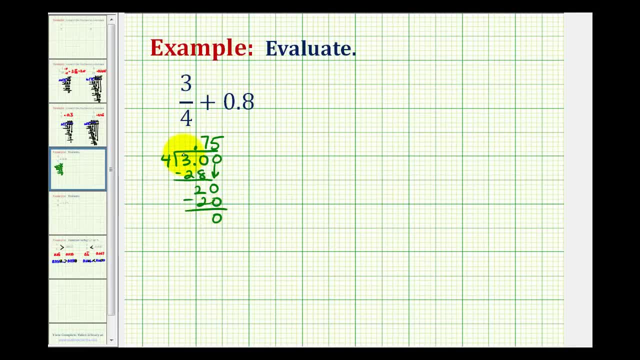 We subtract and we have zero. So three-fourths is equal to zero point seven five. So using decimals, we can write the sum as zero point seven five plus zero point eight. Now to determine the sum using decimals, we would write this sum vertically. 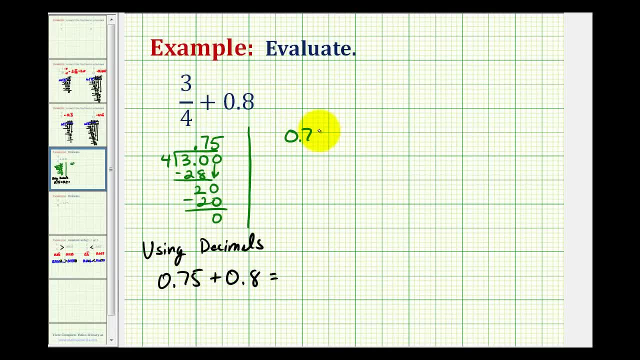 lining up the place values, We would have zero point seven, five plus zero point eight. If we have one or two, we could add a zero in the hundredths place value here, Bring the decimal point straight down and then add as we normally do. 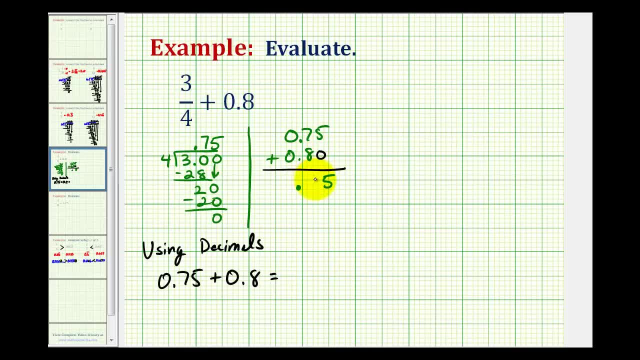 Five plus zero is five. Seven plus eight is fifteen. carry a one. So we have one point five, five or a one in fifty-five hundredths as our sum using decimals. Now let's find the sum using fractions. To do that, we'll have to convert zero point eight to a fraction. 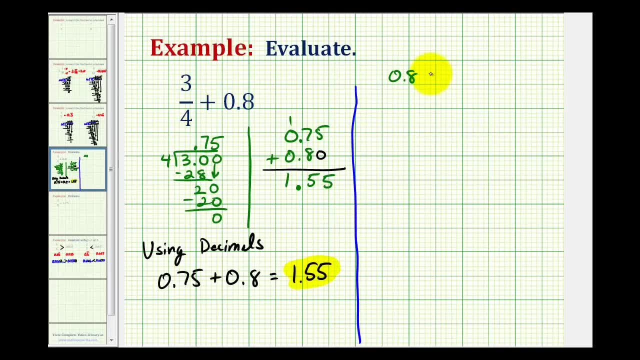 Well, if we know our place values, zero point eight would be read as eight-tenths, which would be eight over ten, Which does simplify. There's a common factor of two between eight and ten, So zero point eight is equal to eight-tenths. 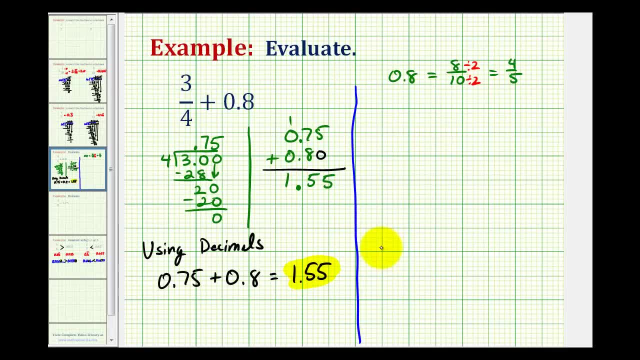 which is equal to four-fifths. So using fractions we could write this as three-fourths plus four-fifths. To determine the sum in fractions, we know we have to have a common denominator. So if our denominators are four and five, the least common denominator would be twenty.